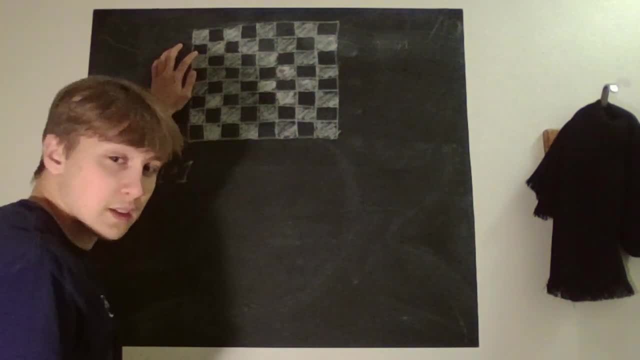 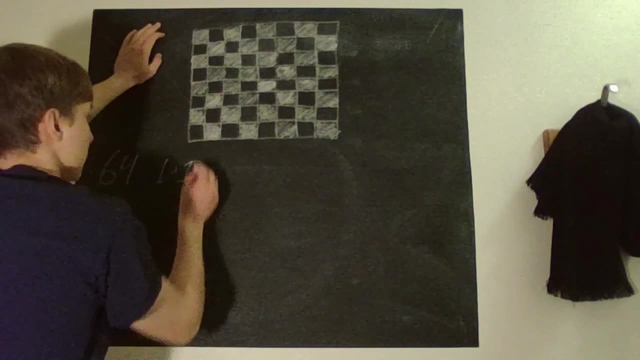 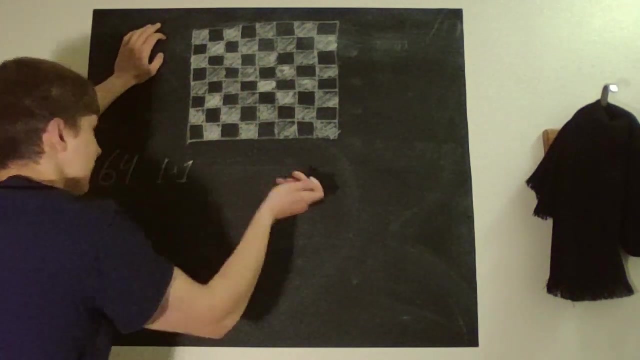 on how many squares can we fit the top left corner? So, okay, we can obviously have it over here. Can we have it over here, though? No, because then the shape would be down here and that we don't allow. So it can't be here, and that means that it can't be on this row. 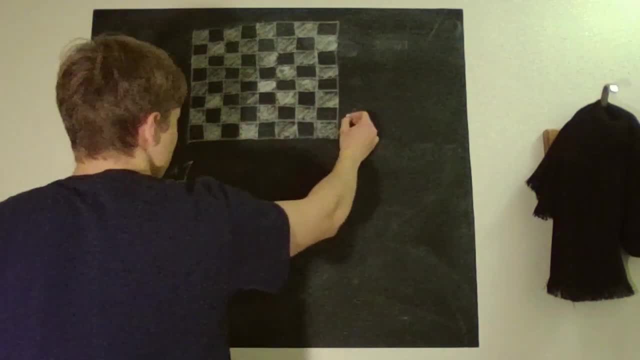 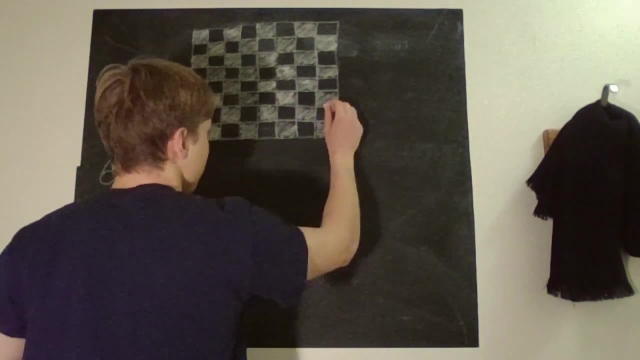 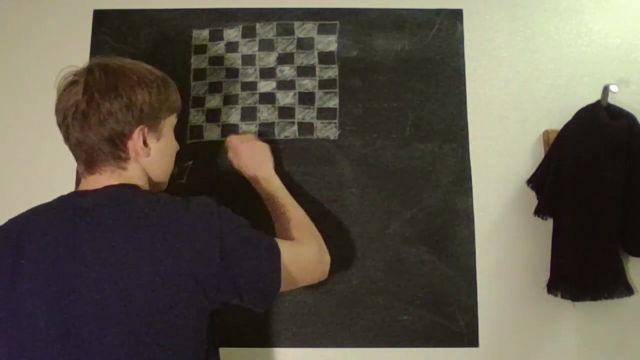 either. So it has to be on this row, And are there any constraints? that way, Well, can we have it over here? No, because then it would be like all the way over here. So the furthest to the right that we can have it is here. Okay, so the top left. 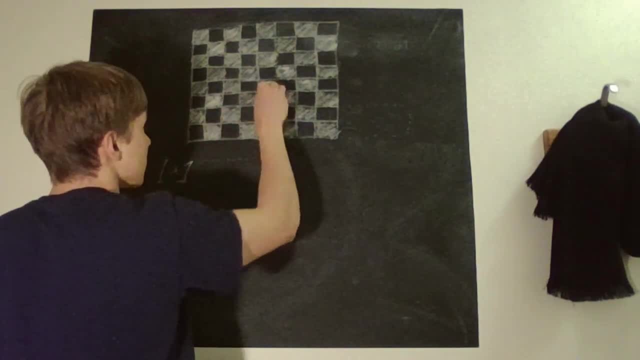 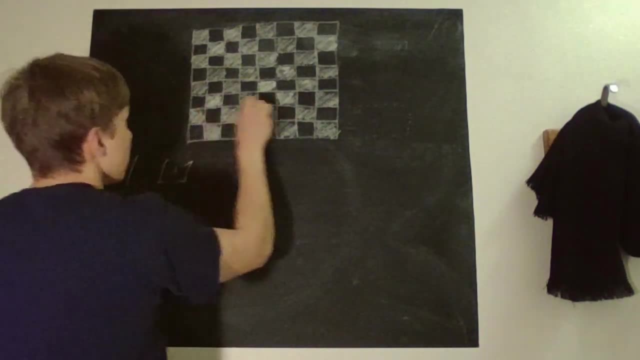 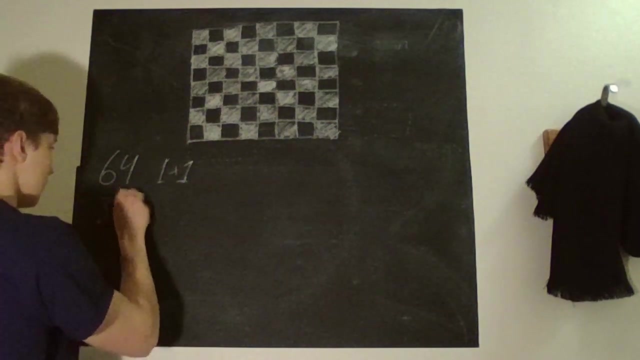 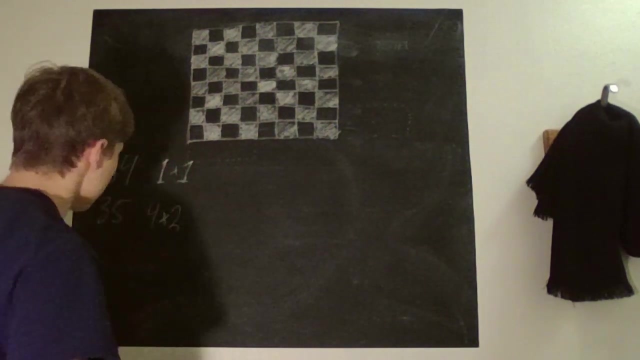 corridor can be, in these squares, in this area, here, and how many of those are there? well, there's okay, it's five times seven. so this, this 35, okay, so we can just write that down. uh, we say 35 four times two ones, and what do we have here? what is 35? 35 is seven times five. 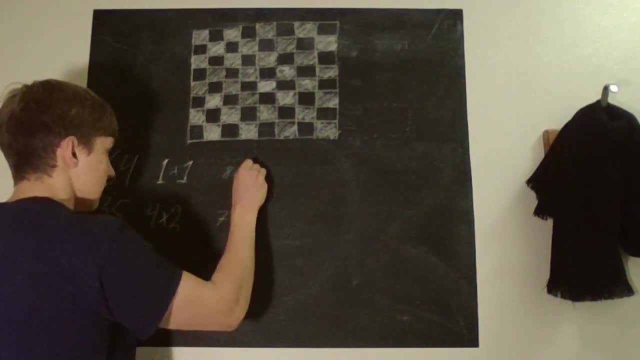 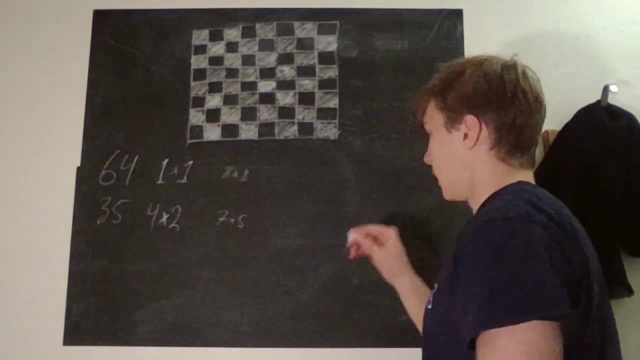 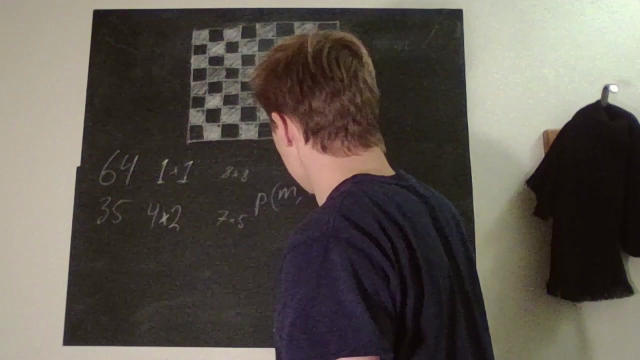 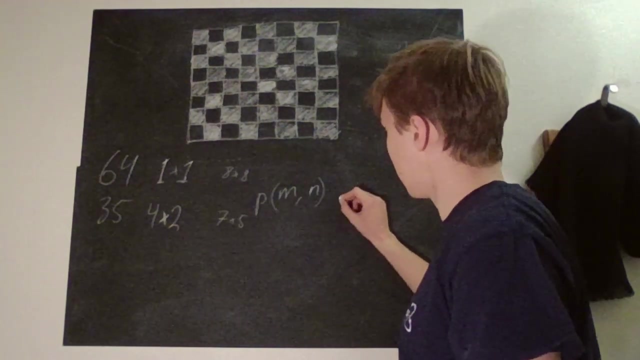 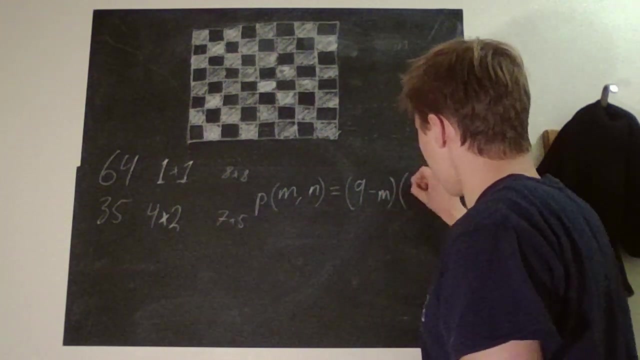 and there are 68 and that was eight times eight. and then we have a one one and a four two. is it possible that a shape with size, say m and m- okay, we have all possible locations- possible locations of a shape with size m and n is equal to nine minus m times nine minus n. 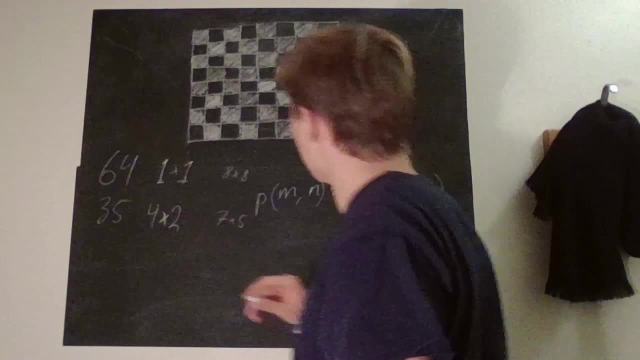 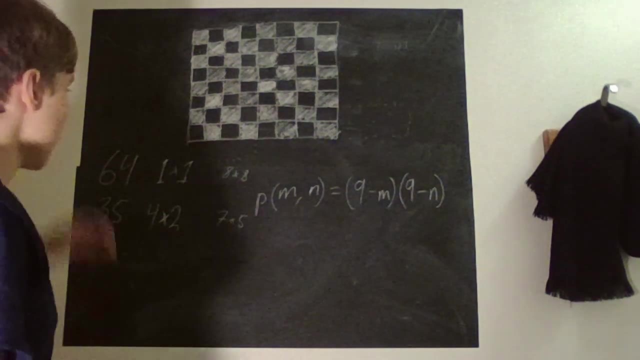 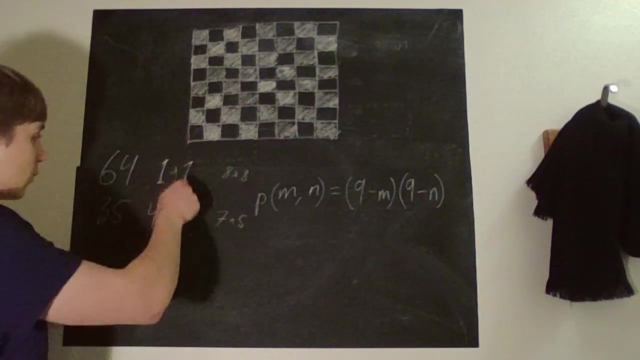 g, which we wanna do. think about this for a while, if you want to, but it should, after a while at least, make perfect sense, because what we have is that, okay, we restrict, we restrict the top left corner with the sizes of the shape, and if it's one wide, then it can fit anywhere. so essentially, we're counting. 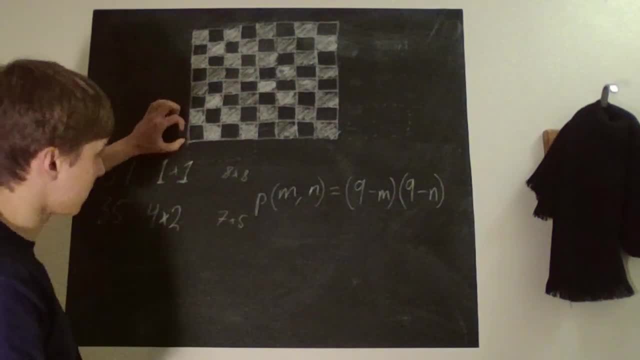 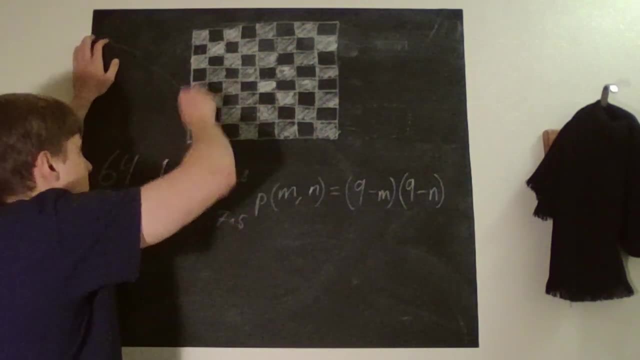 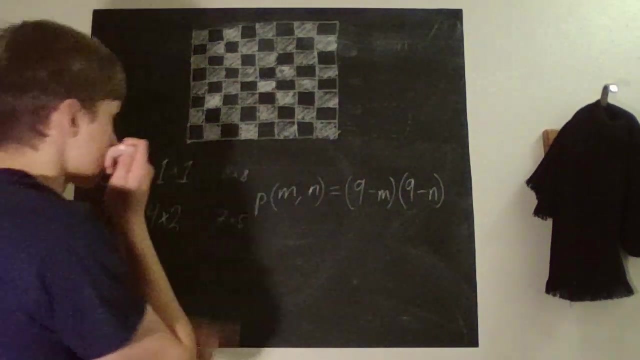 not really counting the squares, more like counting the lines in between, and there's nine of them. so then it kind of makes more sense. you could consider the top left corner- where could the top left corner be? and consider these intersections instead. then it kind of makes up, makes more sense. 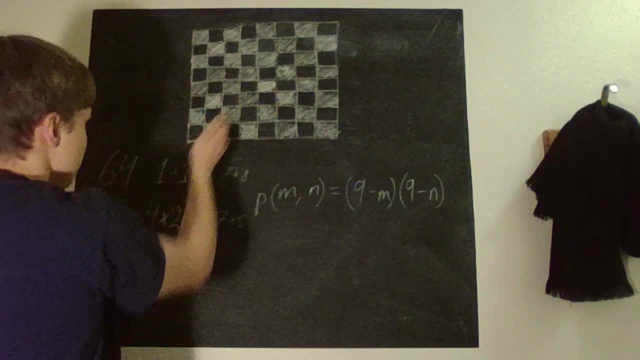 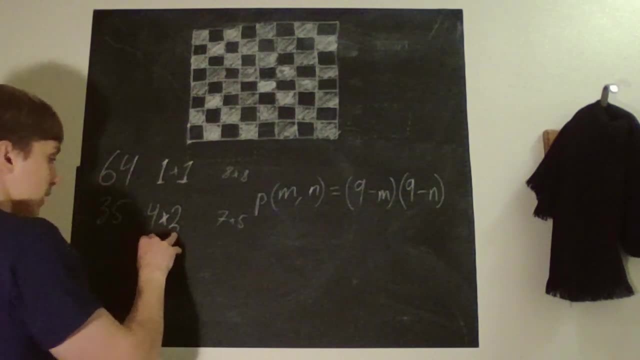 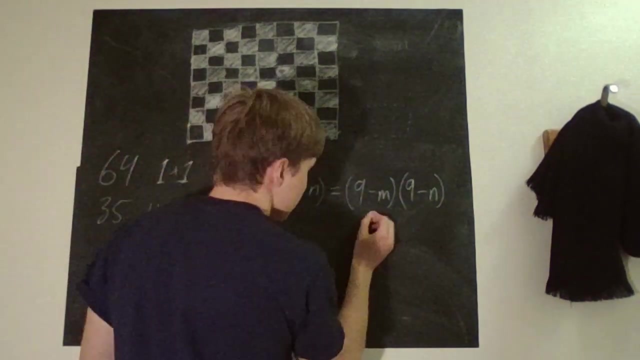 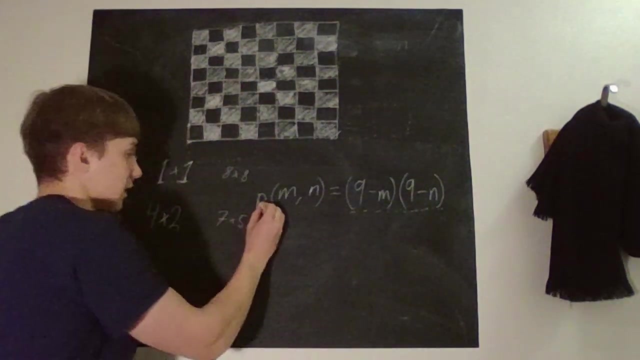 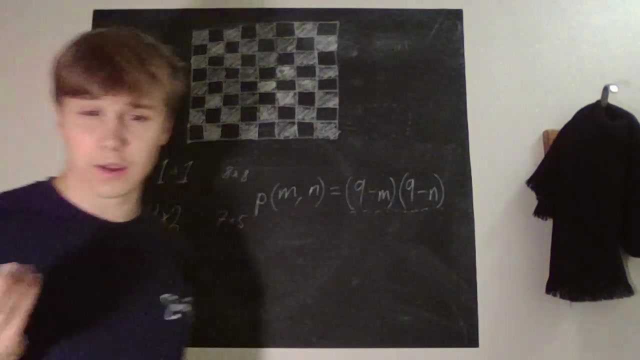 because there's nine lines and but only eight squares. so, as said, we're constraining ourselves with the width and the length of the shape. so this is the formula for how many, how many rectangles there are of the shape m, n, and then we just have to ask ourselves: 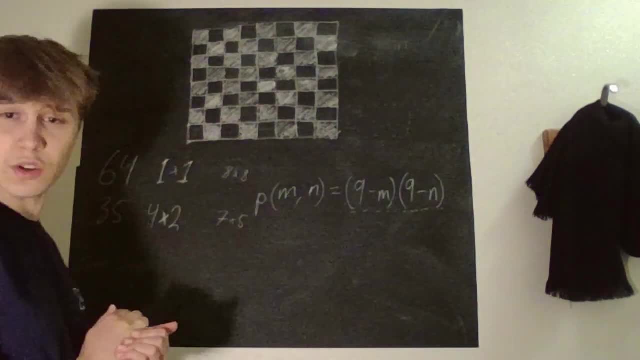 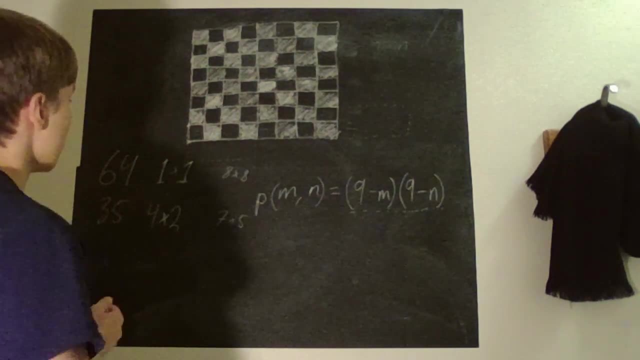 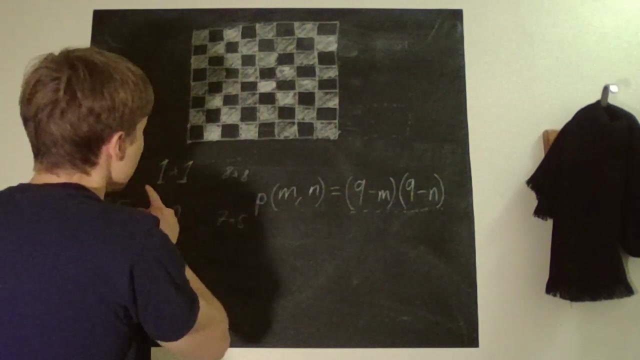 how many shapes are there? well, it isn't. it isn't that hard to figure out. we have the. the smallest we can do is one by one and the biggest we can do is eight by eight. and if we just plug this in here to just check, okay, if it were, if it would be eight by eight. 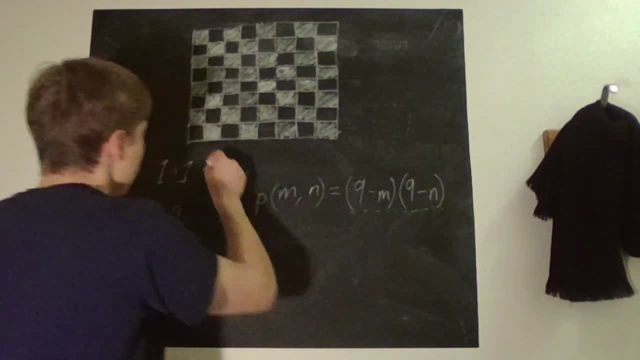 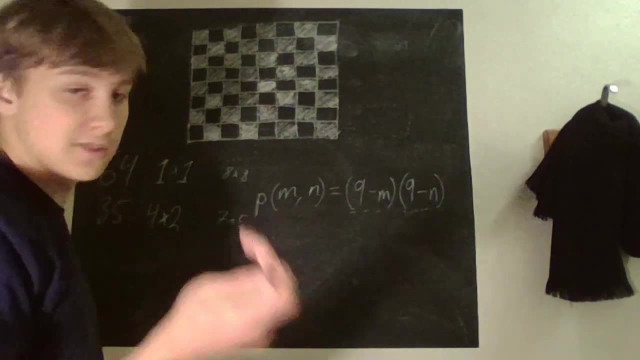 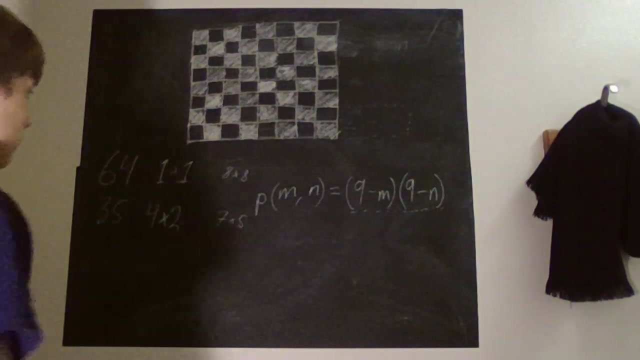 then we have, okay, nine minus eight one, so we have one way, and that is obviously the entire square, the entire board is the eight by eight shape. so what do we get? well, we get a sum because, okay, so we have that for every possible shape we have. 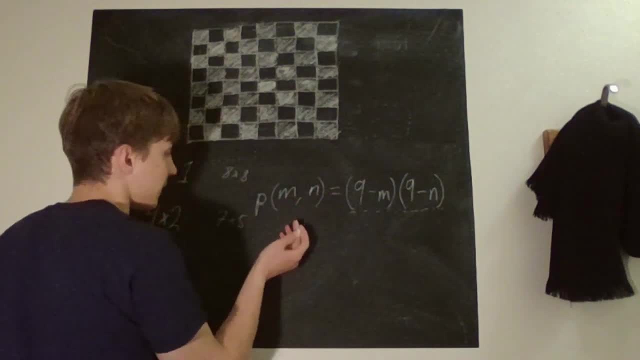 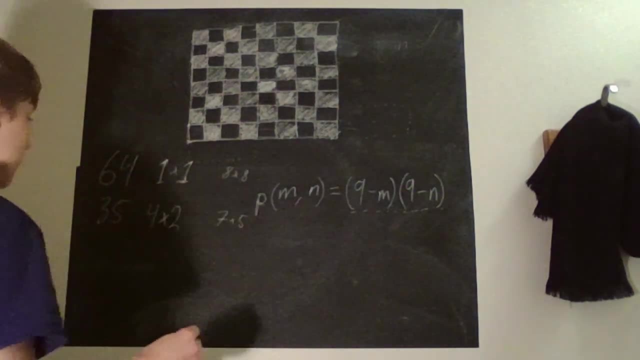 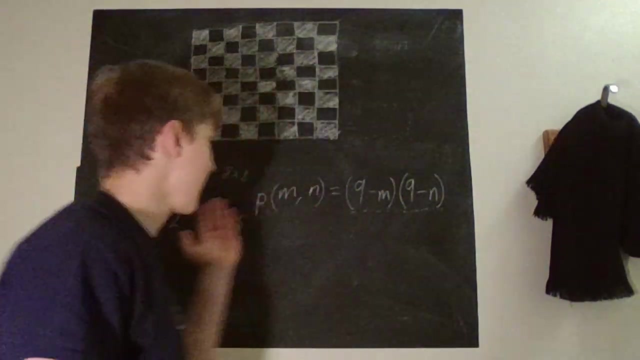 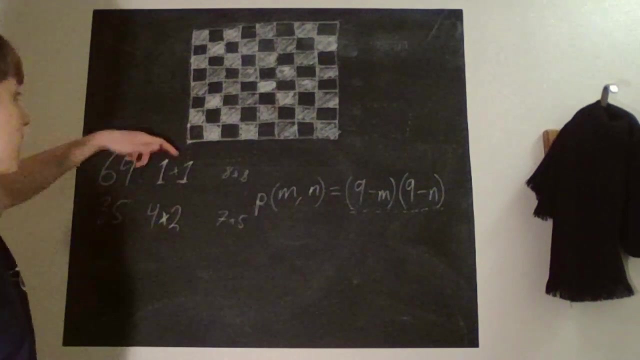 p of m and n possible locations for every which makes a new rectangle. one could say so. we just want to consider every possible shape. so therefore, we have to consider every possible length, which is 1 to 8, and every possible width, which is also 1 to 8. so and then we just sum these up. 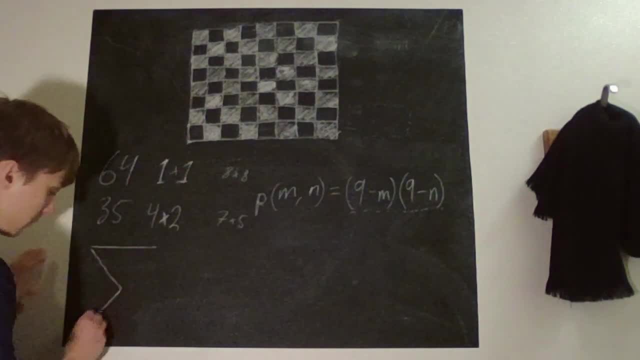 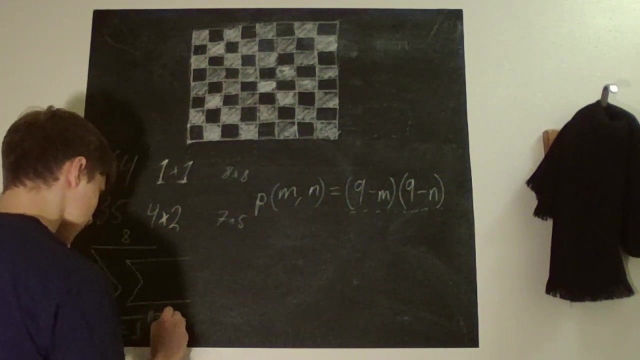 so what do we get? we get a outside sum where m goes from 1 to 8, uh, and an inside sound because we want every single combination of n goes from 1 to 8, of p, of m and n. and now generally a good thing to think about when 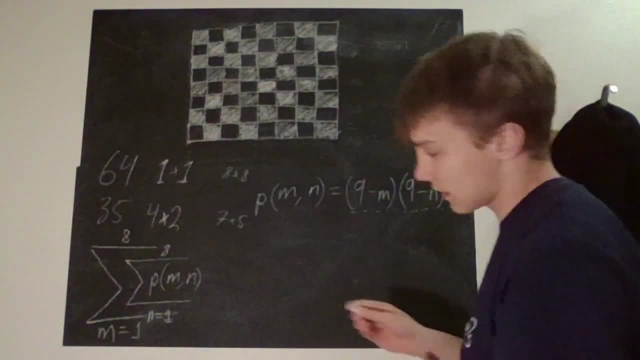 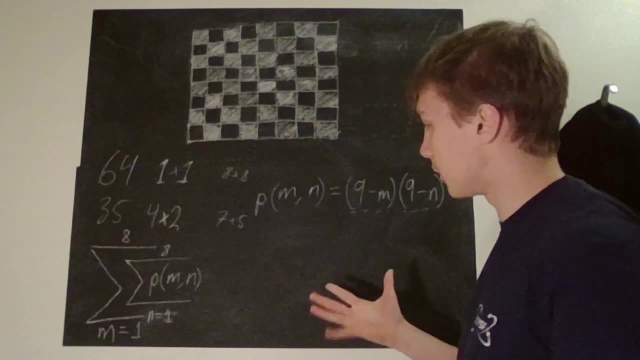 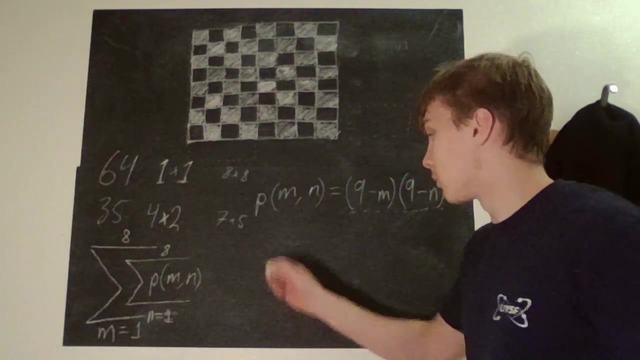 you have these kinds of kinds of things is okay. are we really counting combinations or permutations? or if, what is, what is it we're actually doing? so when we have this, we very much can have the case. we will both have like p of one and two, but we'll also have 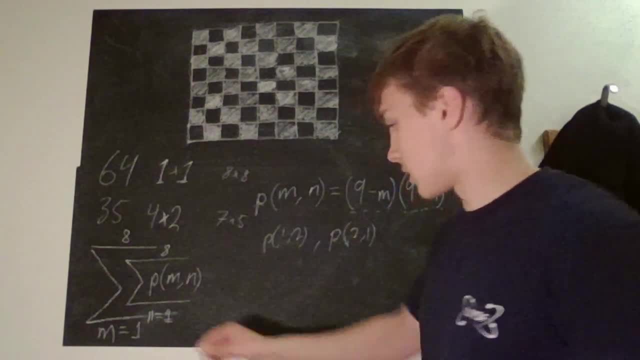 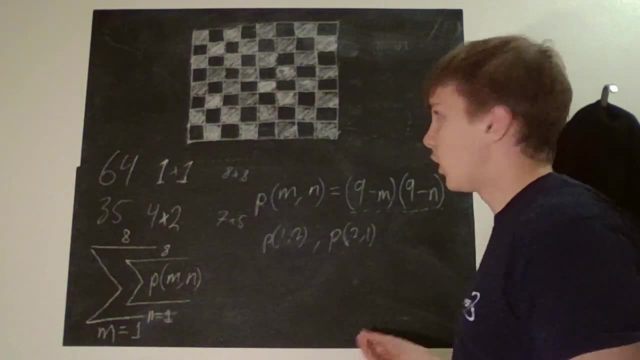 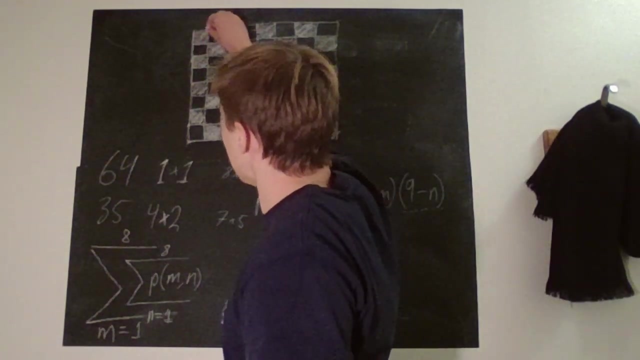 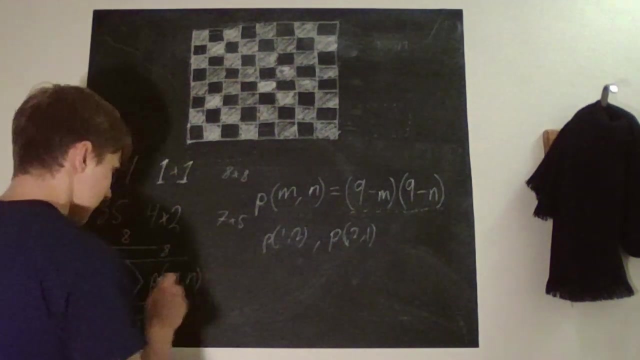 p of two and one, because they, they run through every single combination. so, and is this wrong? no, it isn't, because this is just two by one, that's this shape, and one by two is this shape, or vice versa, whatever you, whatever you want to believe, um so, and this thing we knew was: 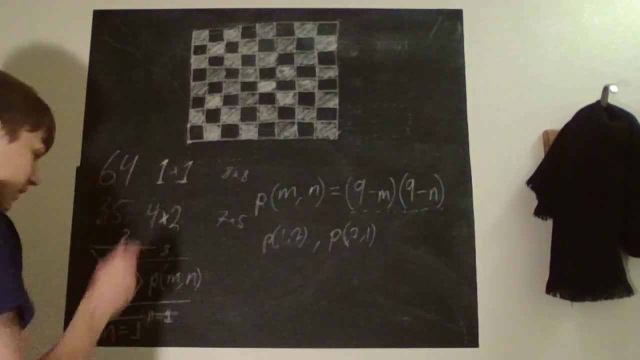 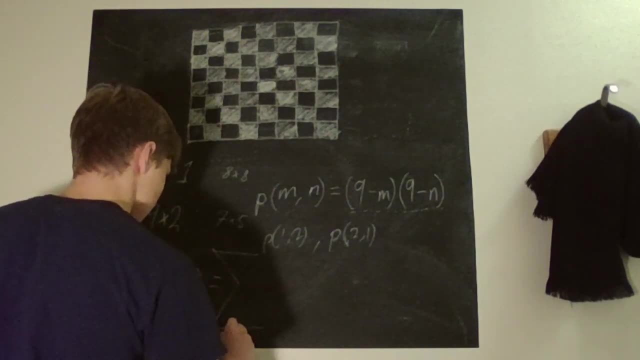 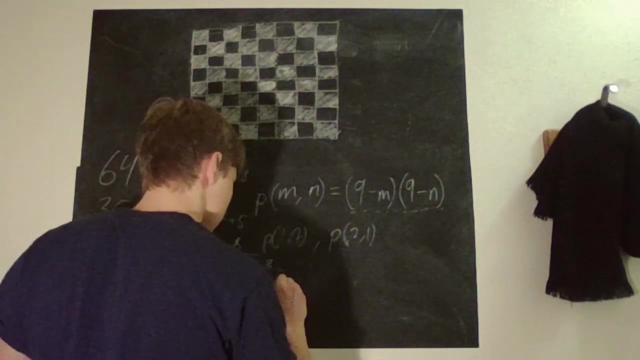 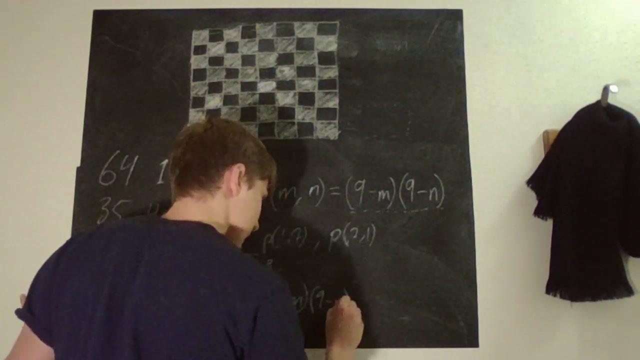 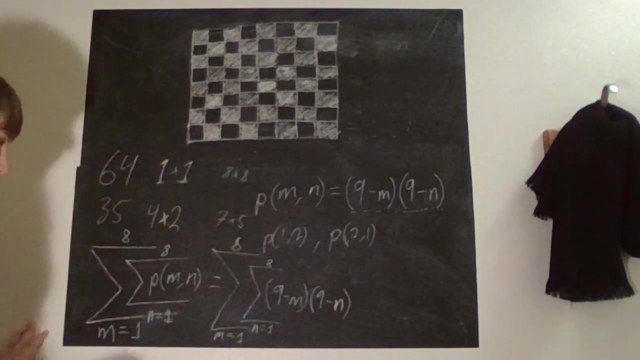 nine minus m and nine minus n. so yeah, we can just write that out again: m goes from one to eight and n goes from one to eight, of nine minus m times nine minus m. and here, if this seems complicated, it really really isn't, but you have to think of it. 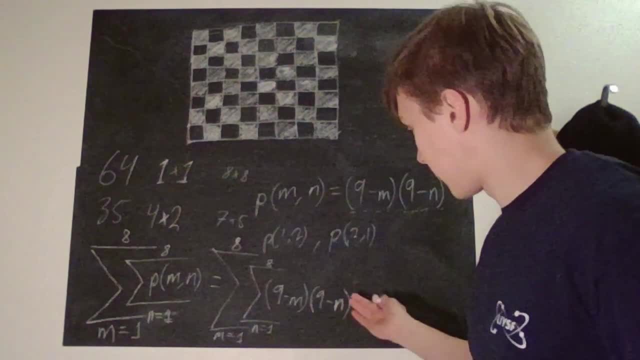 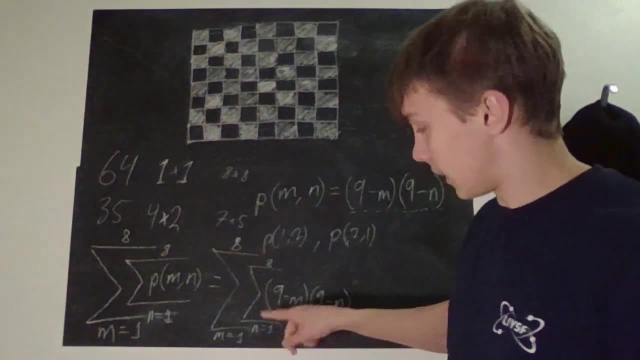 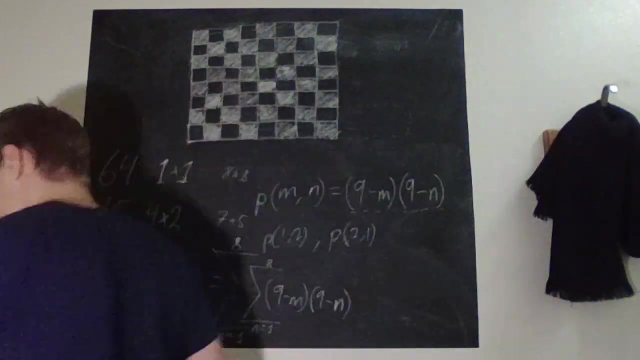 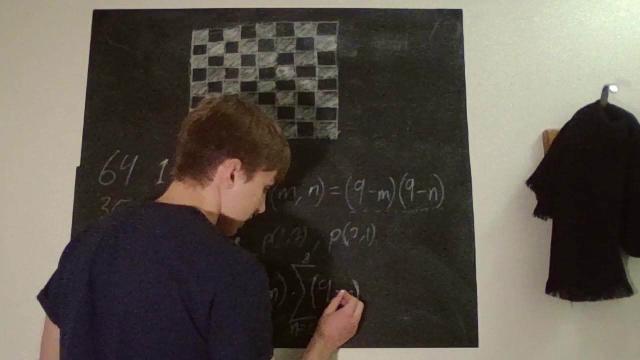 so sadly. so what is this? well, firstly, we can extract this factor from the n sum, because that has nothing to do with n, so we can move that outside. i'll do that real quick. so what is this? okay, this is the sum of: okay, we have eight plus seven plus six plus five plus four. 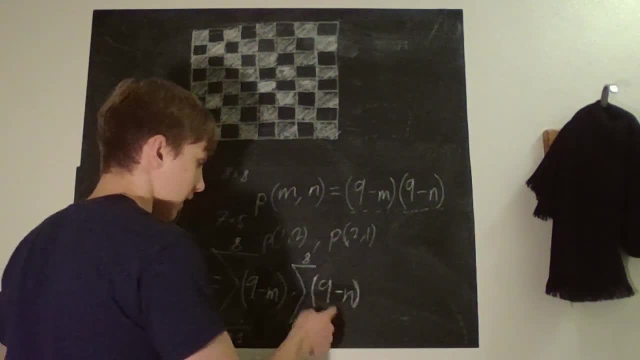 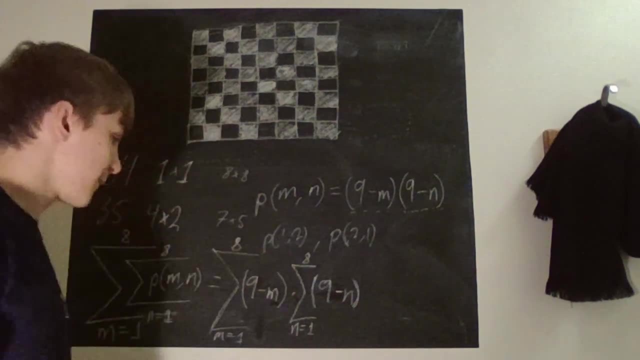 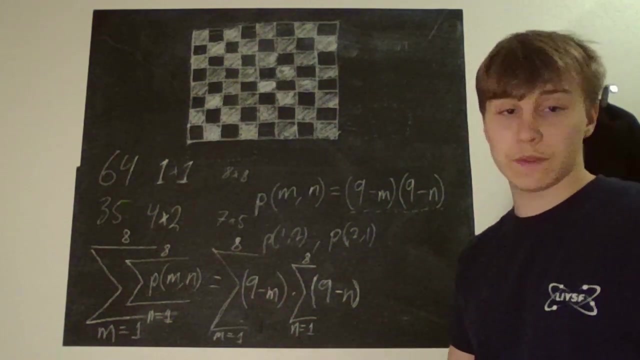 plus three plus four, three plus two plus one. yeah, that's all we have here, and we this, and we have the same here thing here, except we have that with a multiplication. so what is this sum? as i said, it's eight plus seven plus six plus five, which is, and so on, which is just the same. 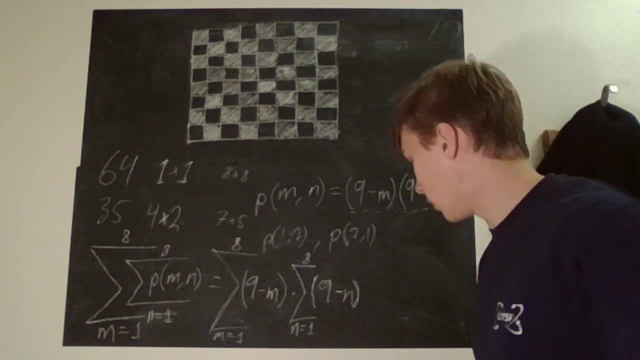 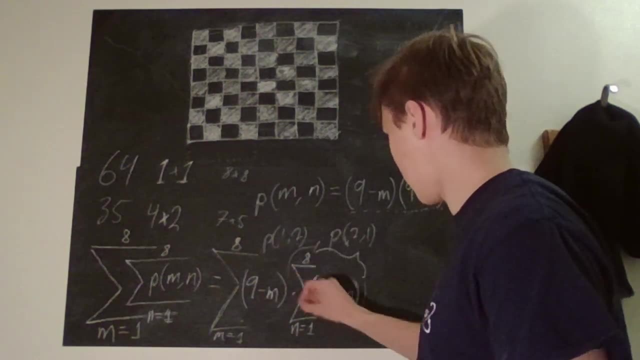 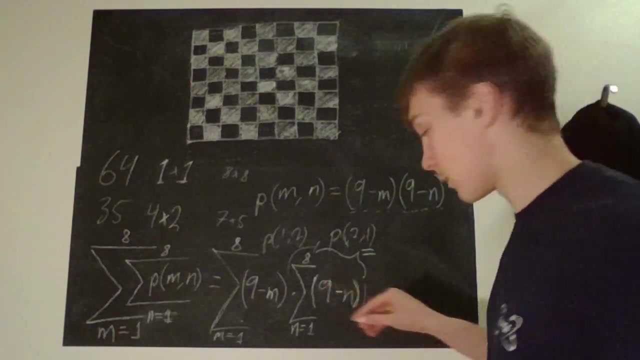 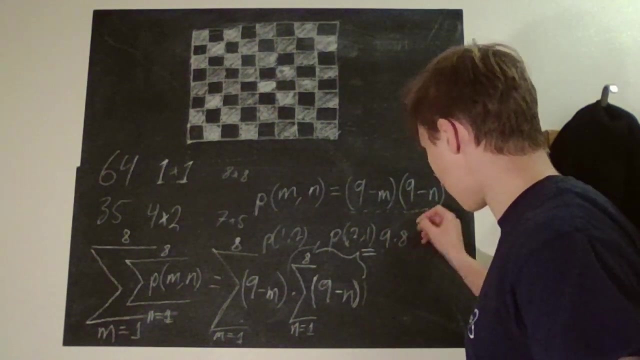 as one plus two plus three, up to eight. and we know that this thing specifically like this here, this is equal to: i think you have seen there a rhythmic sum formula before. so this is nine times eight, because we're going up to eight divided by two, which is equal to 36. 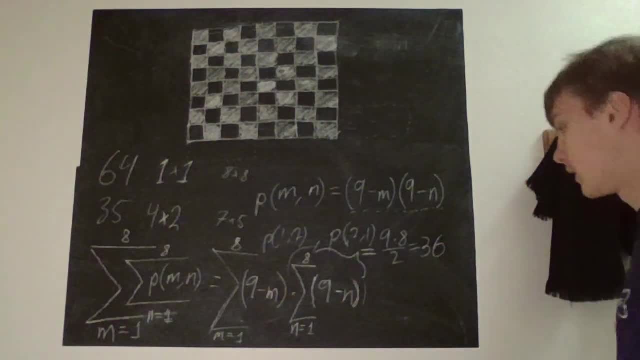 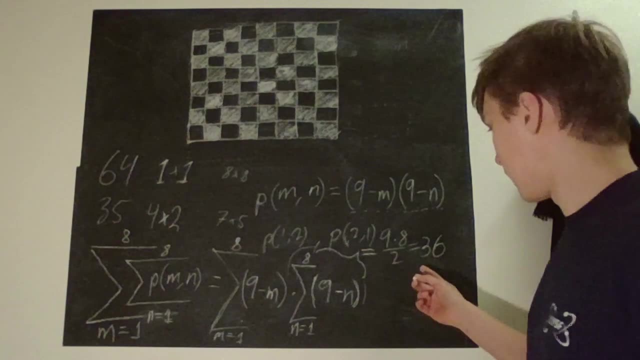 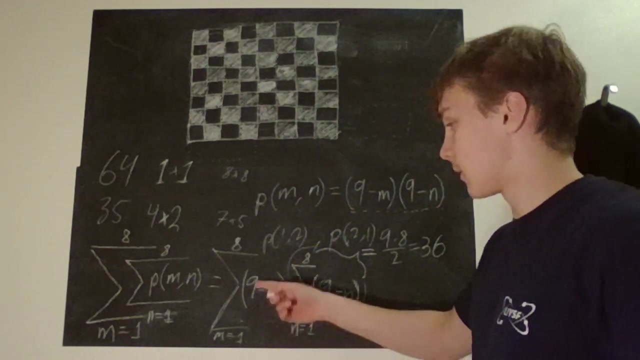 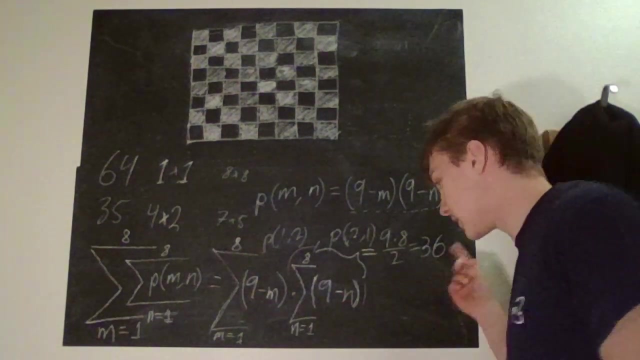 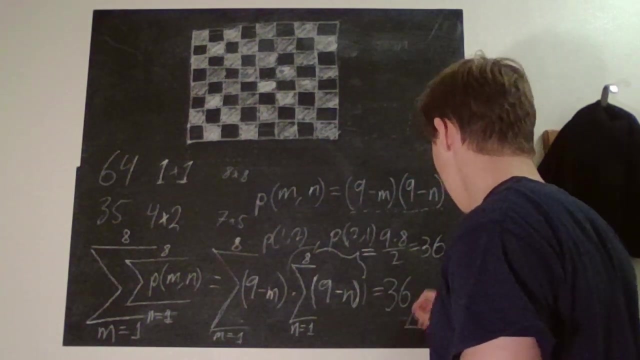 yes, i am correct, 36. so, and that's just a constant. so then we have that. okay, this is okay. the sum of eight, eight, seven, six, five, all the way down to one, all of them times 36, so we can just extract that in front. so we have 36 times the sum of where m goes from one to eight. 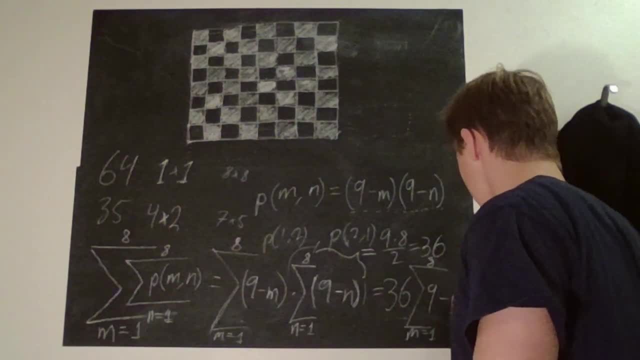 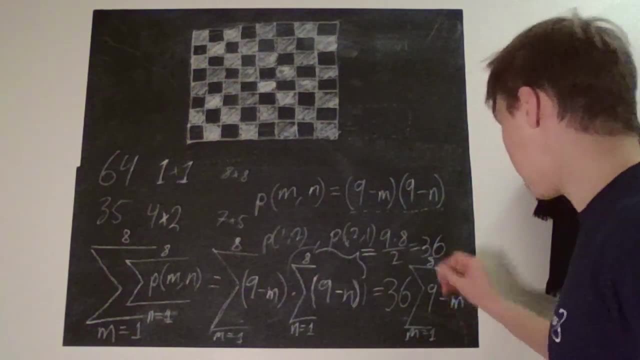 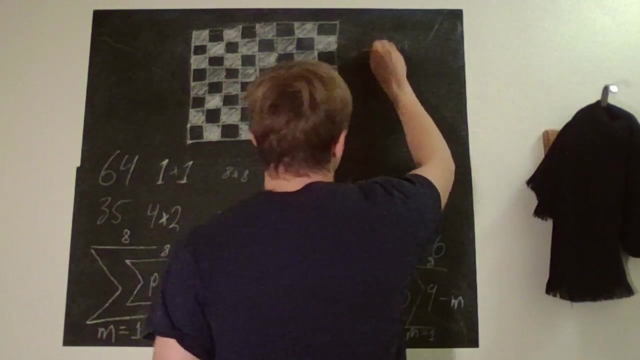 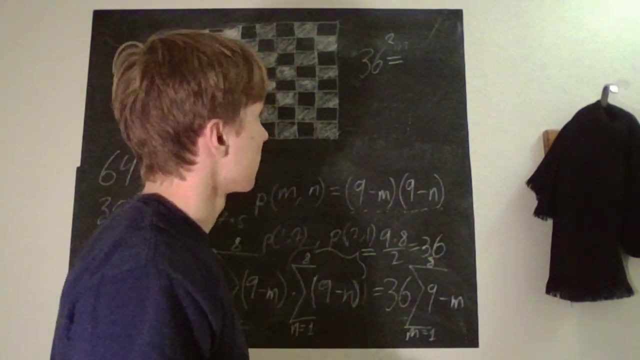 of nine minus m and this thing. that's just the same, because we're just changing the dummy variable. it doesn't make any difference. so this is just also 36.. so our answer is: 36 squared, which is equal to this should be 1296. 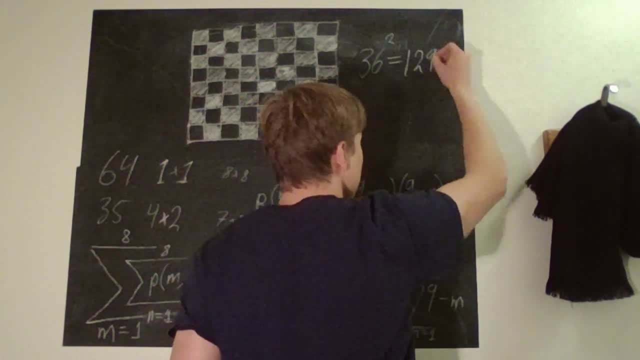 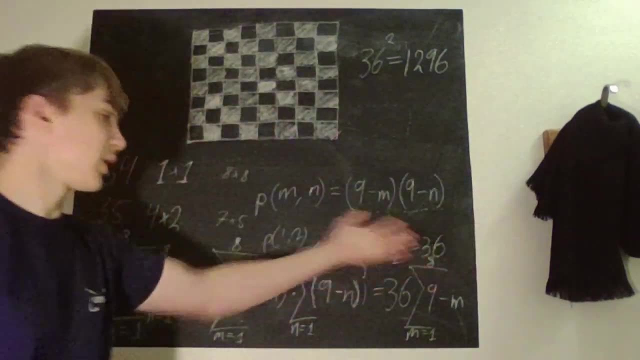 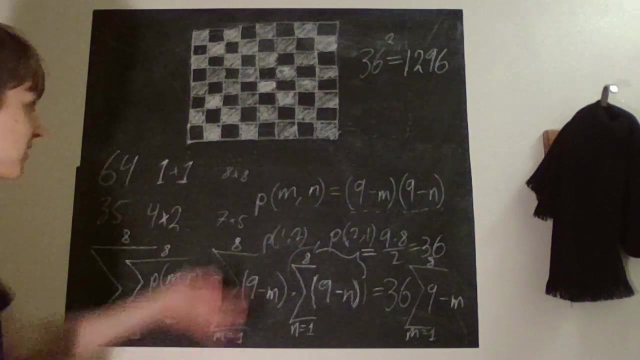 so we have 36 and if that number is correct, i'm maybe bad counting, but that doesn't really, that doesn't really matter. you can look it up. we've, we've, we've done the process. okay, we've done the process. so yeah, um, so this is, this is the answer, and i can just recap the method real quick.